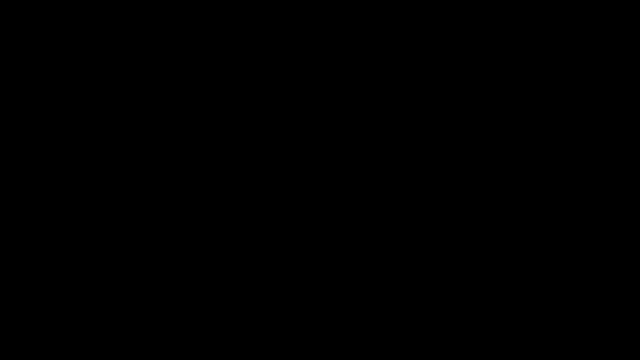 Usability testing with the ThinkAloud protocol is widely used in the industry. In these test sessions, participants verbalize their thoughts while performing actions on the user interface. However, analyzing large amounts of these recorded sessions is time-consuming. It's also susceptible to the evaluator effect, where multiple people identify different problems for the same interface from the same user session. 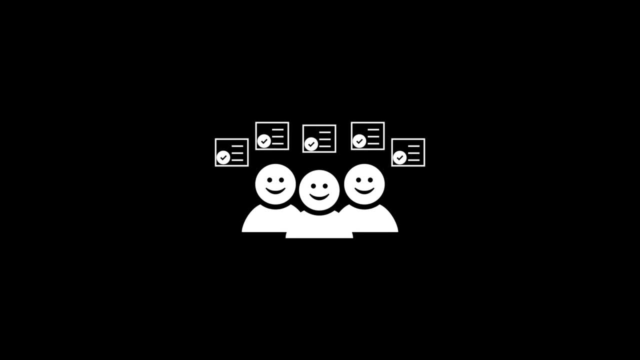 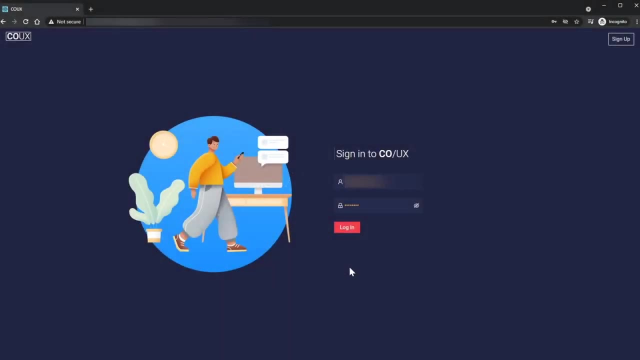 which is why collaboration is so important in data analysis. We built a collaborative visual analytics tool called CoUX to support multiple UX evaluators with analyzing ThinkAloud usability test recordings. Emma is a UX evaluator who would like to use CoUX. She logs in and sees the project overview. 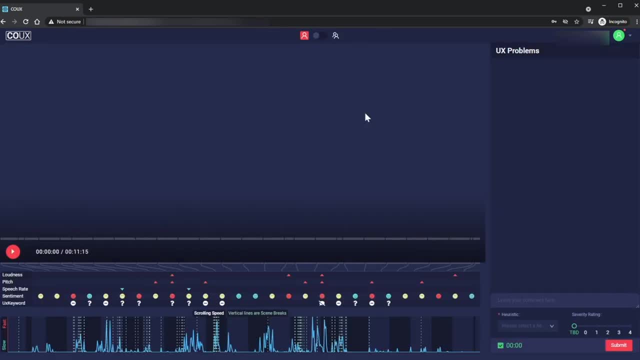 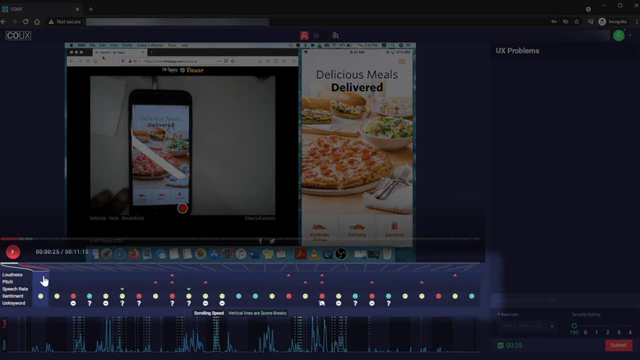 She then selects a video regarding an older adult ordering pizza. Emma sees the video player on the top left of the screen. Below, she sees a feature panel that contains the matrix showing acoustic features like loudness, pitch and speed rate. textual features, including sentiment and UX keywords. 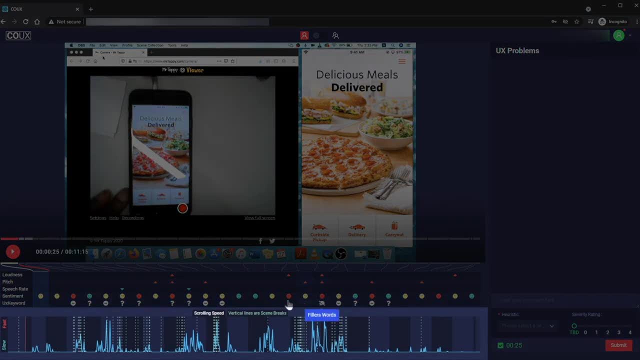 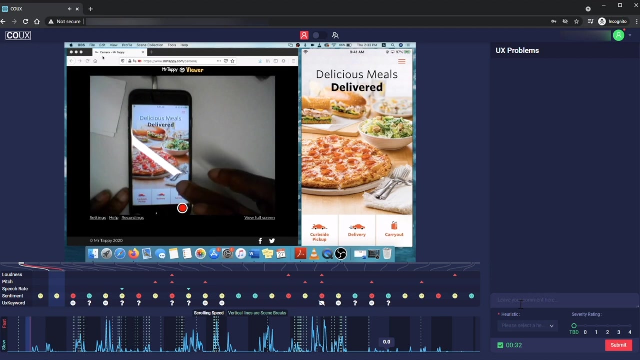 and visual features, including scrolling speed and scene blanks. Now she starts reviewing the video to identify usability problems. When the video is playing a particular segment, its corresponding column on the feature matrix and the graph are highlighted. Emma noticed a usability problem in this segment. 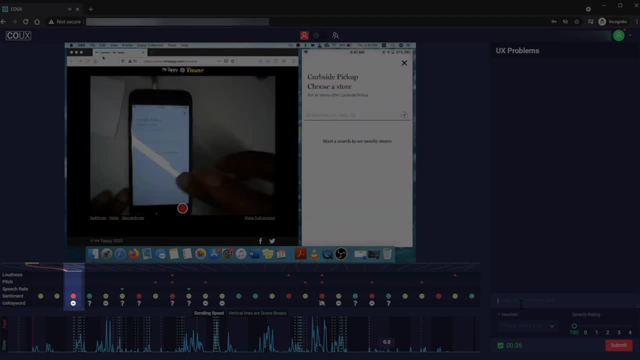 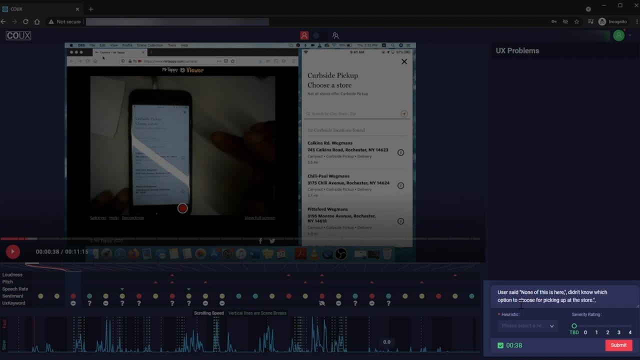 and saw that the sentiment was negative and the UX keywords show the negation signal. She then clicks on the description icon. She types in her description about the user being confused at which option to choose for collecting pizzas at the store. She also selects a heuristic from the dropdown list and adds a severity rating. 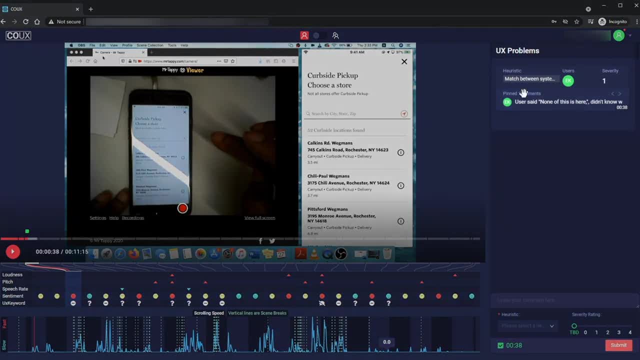 After she presses submit, she sees that the card appears on the annotation panel. A colored square also shows up at the current timestamp above the video progress bar. This gives her an overview of all the annotations that are entered throughout the video. Emma then utilizes the feature panel and reviews the rest of the video. 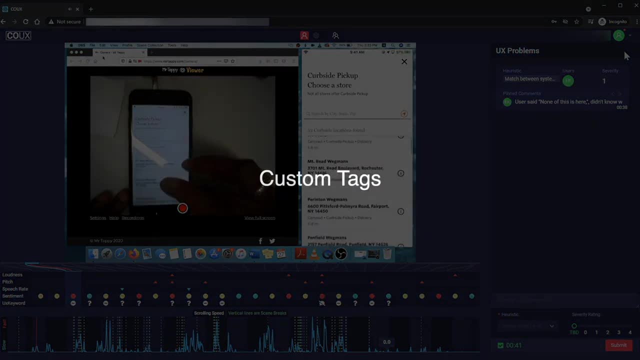 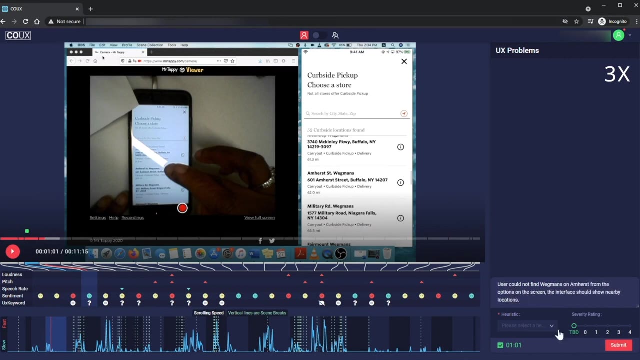 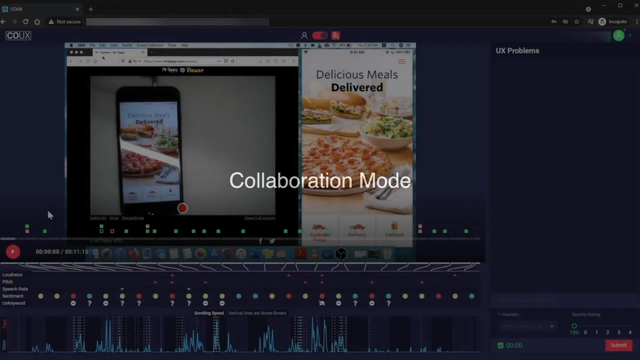 before switching over to collaboration mode, Emma continues her review and finds another problem. Instead of choosing the default heuristics, she can also add a custom tag that is relevant to the problem currently experienced by the user. In collaboration mode, she can view the comments of her partner.